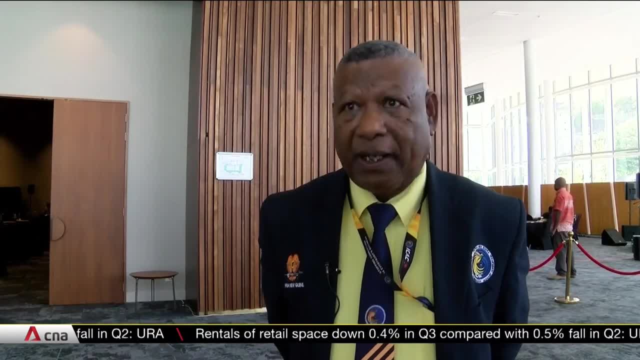 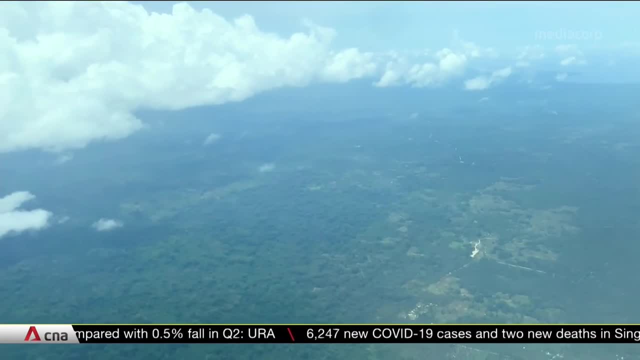 level of corruption that has infiltrated from the very top right down to the little people in the communities. But, in fairness, not everyone rorts the system And for big corporates who abide by the law, there are still extraordinary riches to be made, both above and below ground. 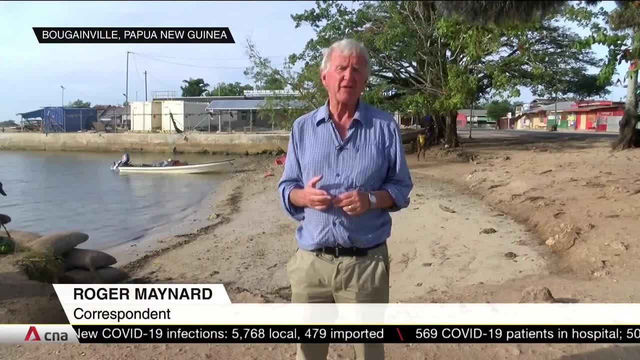 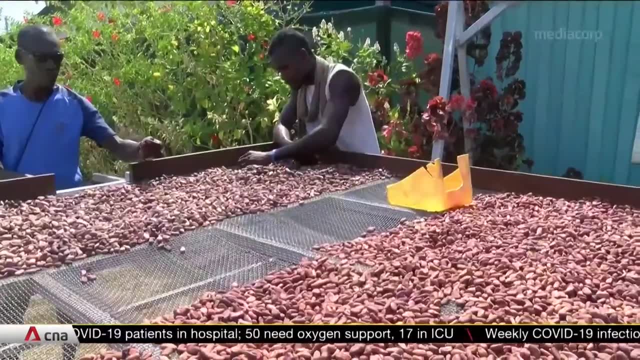 PNG has vast natural resources. It's an Aladdin's cave of minerals, including copper, copper and gold, which are found in such abundancy here in Bougainville. Today, this autonomous region survives on government aid and a largely agrarian economy. 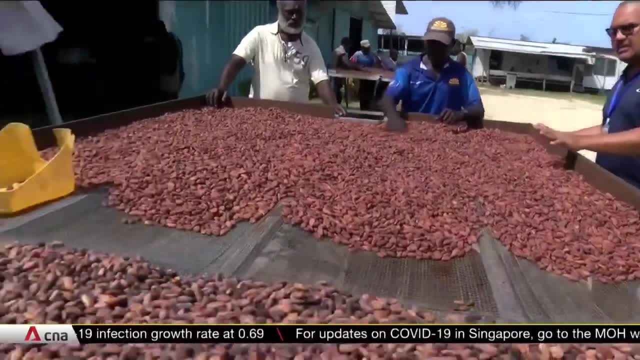 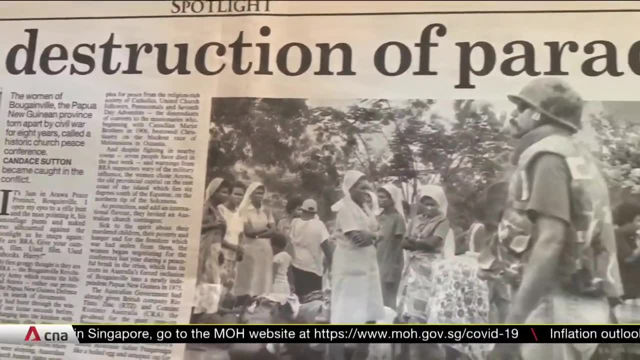 But there was a time when Bougainville boasted one of the world's biggest copper mines, producing massive profits for the owners but little for the community. A civil war which forced the closure of the mine more than 30 years ago claimed 20,000 lives. Now there are hopes. the 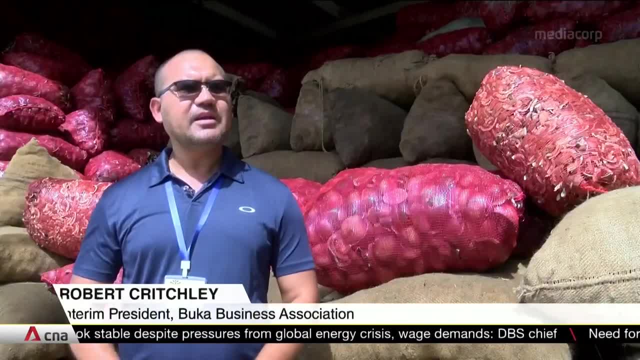 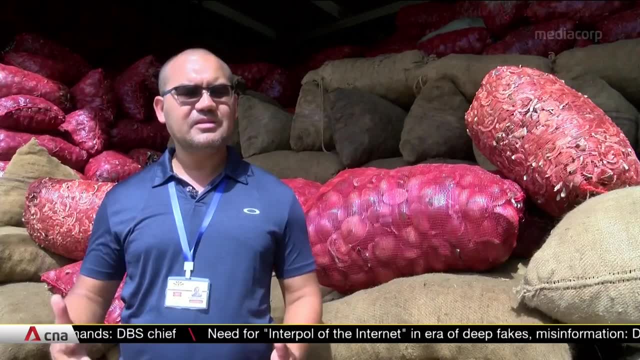 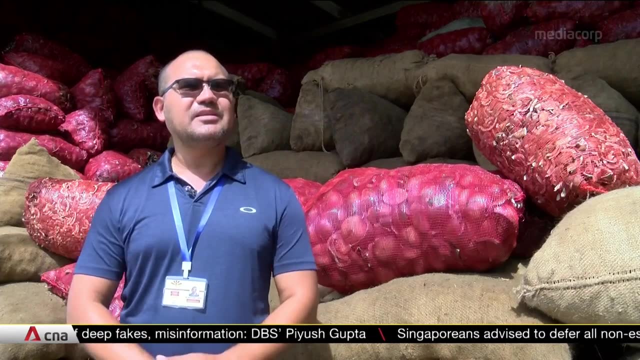 Panguna copper mine could reopen. The PNG mine, which was once the largest copper mine in the world, is now open. In the case of Bougainville, we have a great opportunity in Aachai to do things right, where the indigenous people of Bougainville can get better benefits from whatever is extracted. 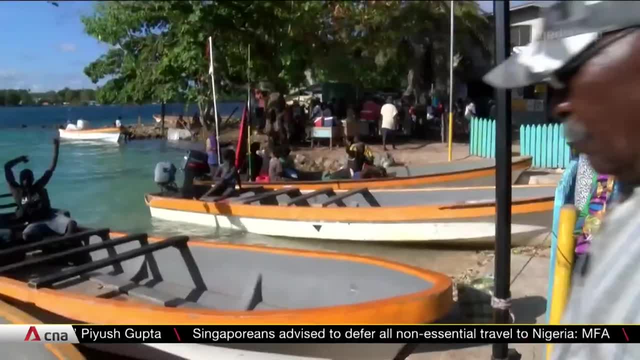 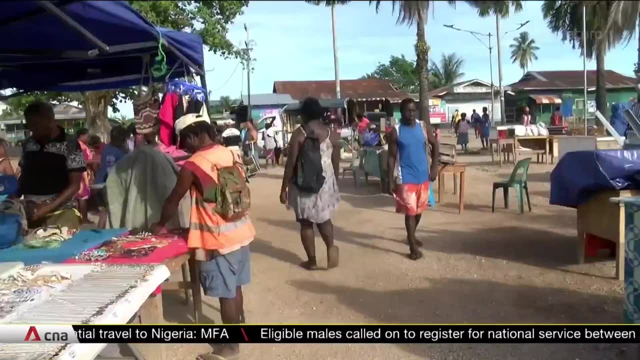 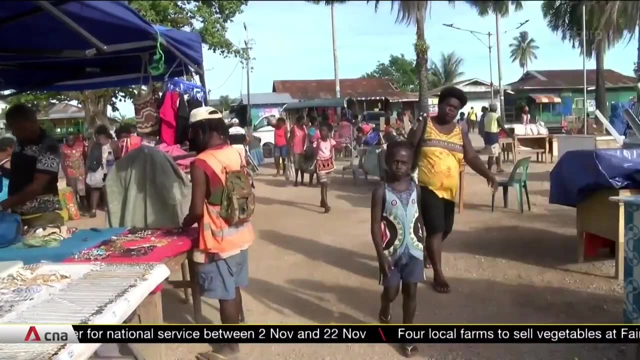 in, But it has to be. a proper plan has to be done. Bougainville's autonomous regional government is also demanding full independence, which was supported by 97.7% of the population in a referendum, But the outcome is far from settled and, in the meantime, the people rely on their modest economy. 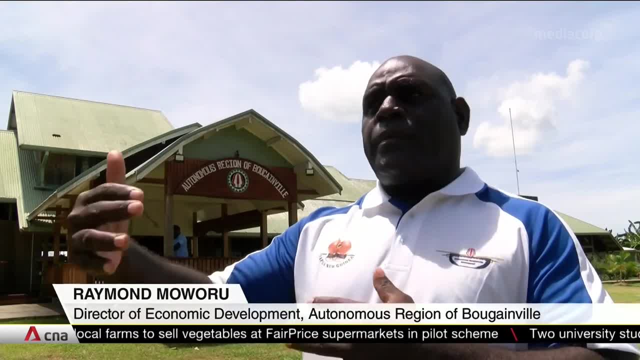 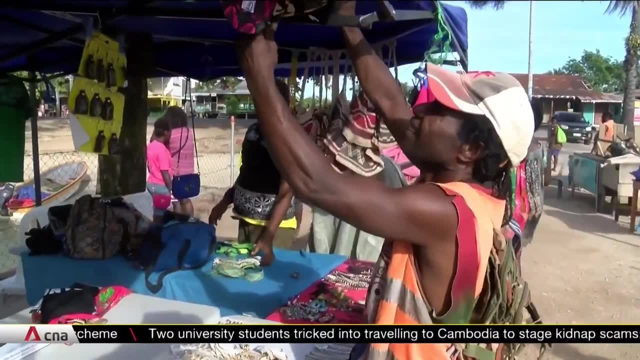 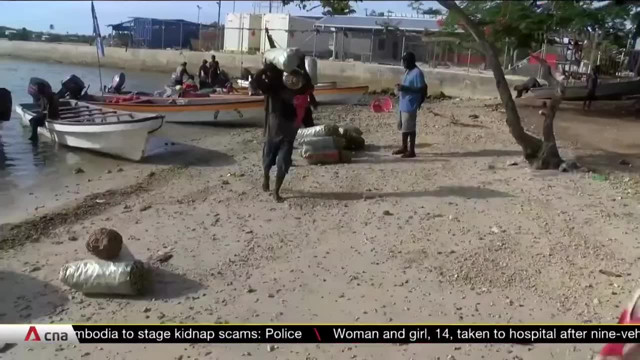 The financial position of Bougainville is very important in terms of sustaining the independence of Bougainville, But independence is by no means assured with the referendum still to be ratified by the PNG government. Even if an agreement is reached, it may take another decade for the lucrative 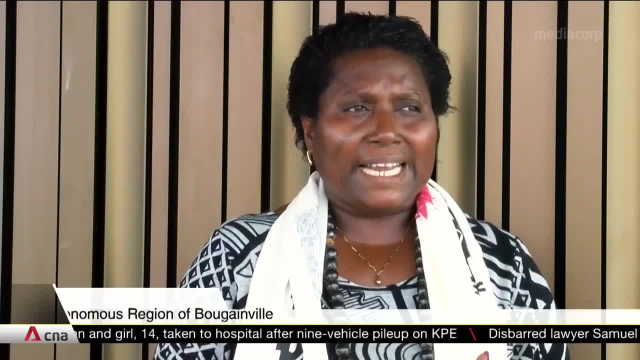 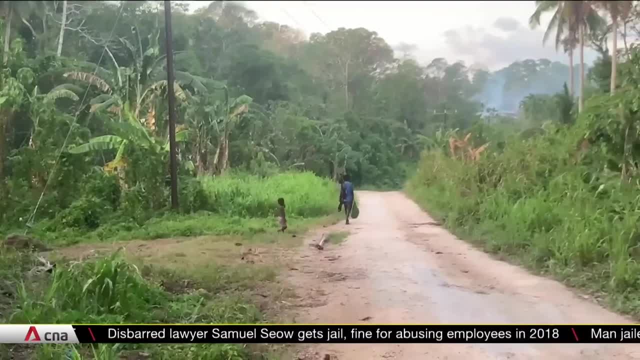 Panguna mine to be cleaned up and reopened. In terms of government's priority. to open the mine, yes, we do, but we have to make sure that we do it right. There's no shortcut. That means a fair share of the profits for landowners and a community that's not divided. 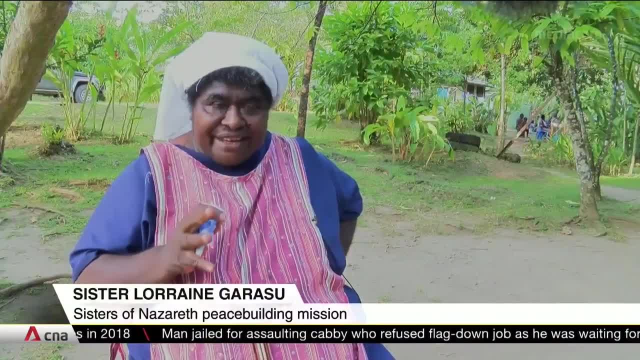 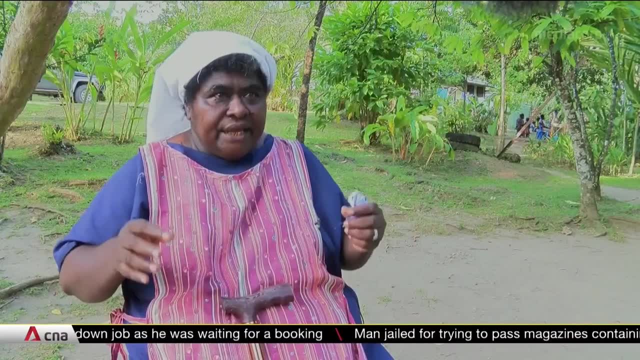 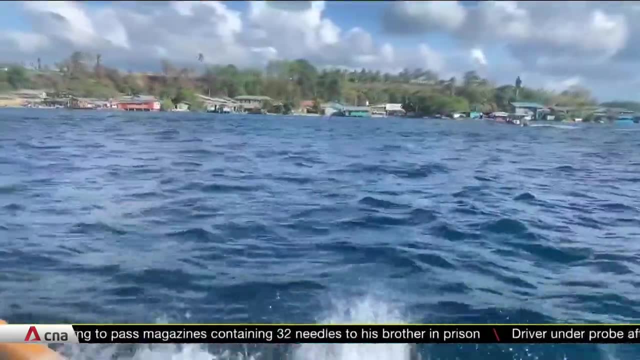 by the violence of the past, Bougainville, within the crisis, became very disintegrated. Many issues, many people died and families were disintegrated, displaced, and all that. Today, Bougainvillians and the rest of PNG look towards a more peaceful and prosperous.